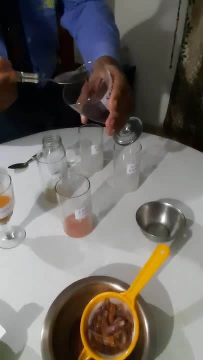 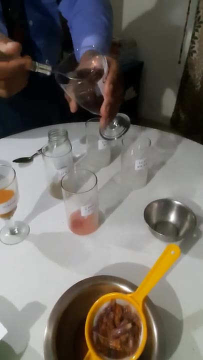 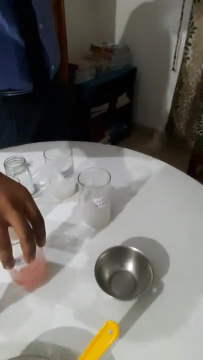 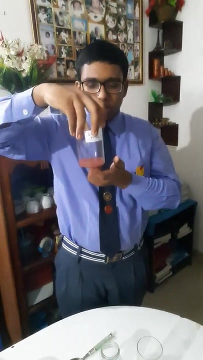 We can observe that the colour of this solution turns to pink. Now I am going to mix this lime juice into this lime juice. 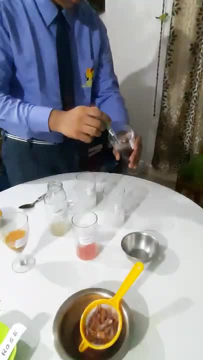 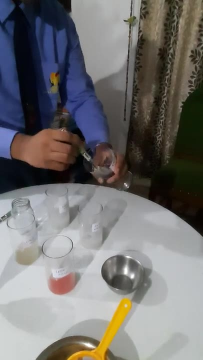 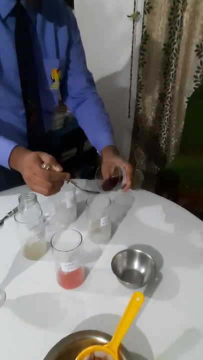 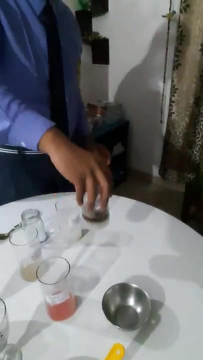 Now I am going to add channel rose water into soap water. I am going to mix two solutions while shaking the glass. 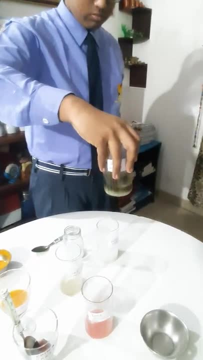 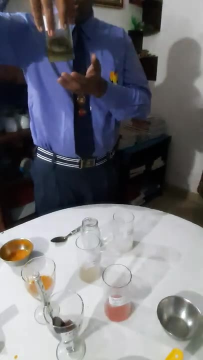 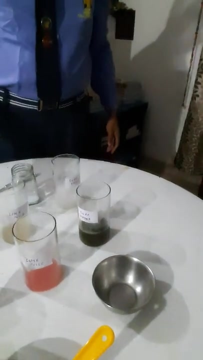 We can observe that soap water solution turns to green. 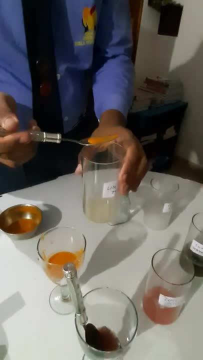 I am going to add turmeric paste into lime juice. Now I am going to mix this lime juice into this lime juice. I am going to mix this lime juice into this lime juice. Now I am going to mix this lime juice into this lime juice. 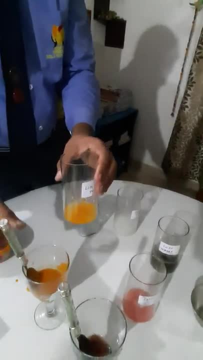 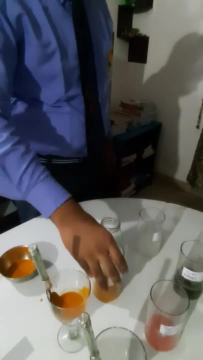 We can observe that mixture of two ingredients is completely mixed. Now I am going to mix two solution carefully. 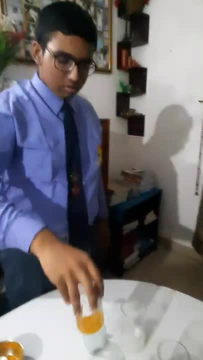 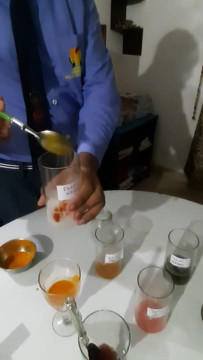 We can observe that the colour of this mixture remains unchanged. I am going to add turmeric paste into this lime juice. Now I am going to add turmeric paste into this lime juice.